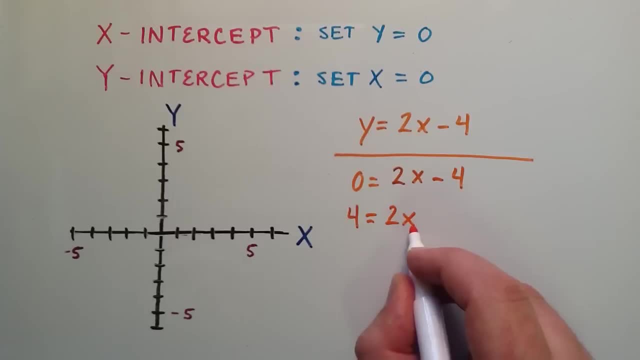 So we're going to solve for x. So now we have: 4 is equal to 2 times x. well, if we divide the left and right hand side by 2, we can get x by itself on the right hand side. So 4 divided by 2 is equal to 2, 2x divided by 2 is equal to x. 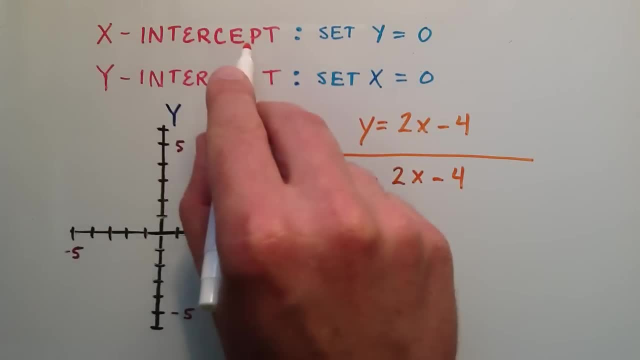 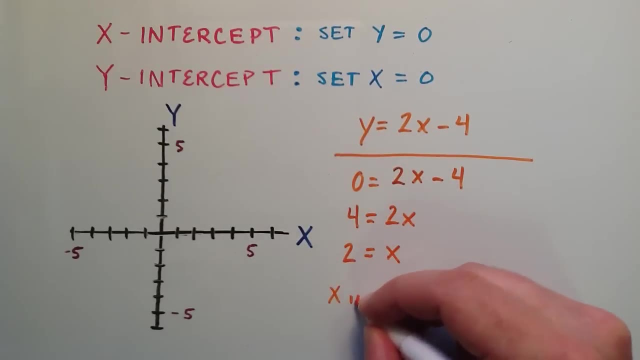 So this is the x component of our x intercept and we know that our y component is equal to 0. So our x intercept- let's go ahead and write this down- x intercept is basically going to be an ordered pair and remember, an ordered pair has just an x component and a y component. 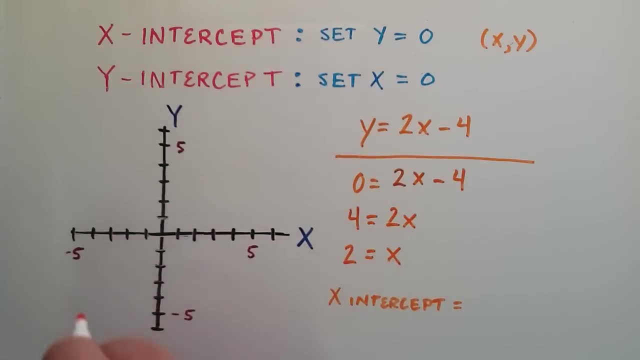 and an ordered pair makes up a point in the xy coordinate system. So the x intercept is going to be the point represented by the x component of 2 and a y component of 0.. Okay, So this is the x intercept of our line, right here. 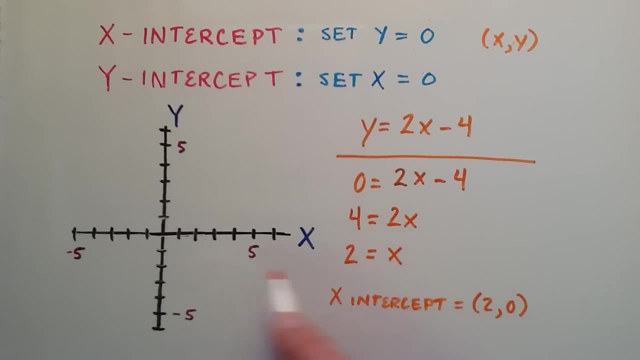 So let's go ahead and just plot this really quick. So on the x axis, when y is equal to 0, that's basically the x axis. so that's our x component is somewhere along the x axis, that's y is equal to 0.. 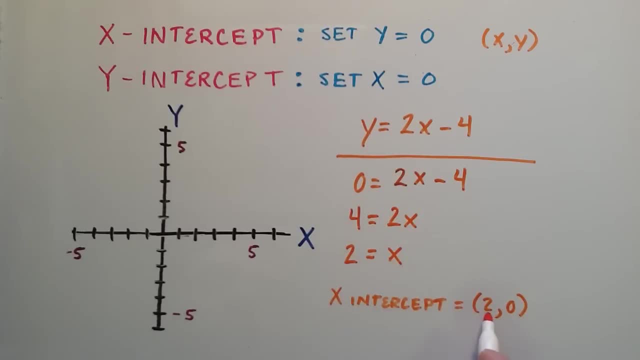 And then x basically is equal to 2, so our x component is 2.. So the point is right here. So that is the x intercept of this line. So let's go ahead and find the y intercept of our line now. So basically, to find the y intercept, we're basically just going to do the same kind of 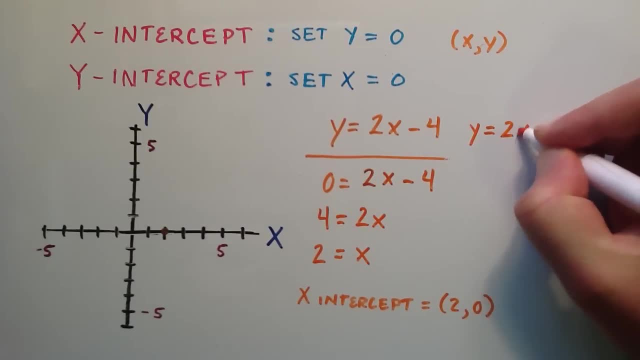 process We're going to be looking at. y is equal to 2x minus 4, once again, just kind of rewrite it here and just kind of work side by side. So this time we're going to find the y intercept, So we're going to set x equal to 0. 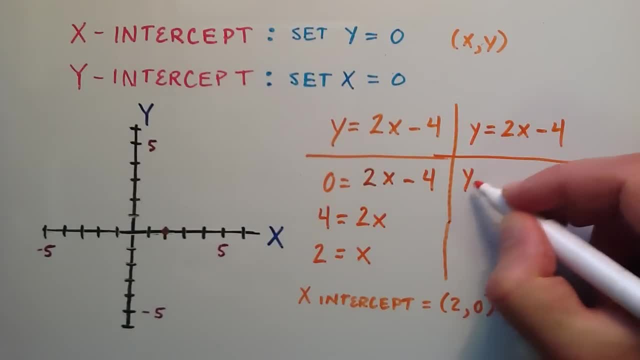 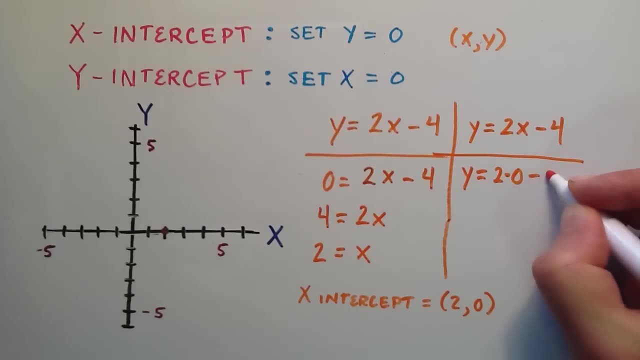 So we're just going to rewrite this: y is equal to 2 times x, but x is going to be 0. So 2 times 0 minus 4.. And anything times 0 is just simply 0. So y is equal to 0 minus 4..